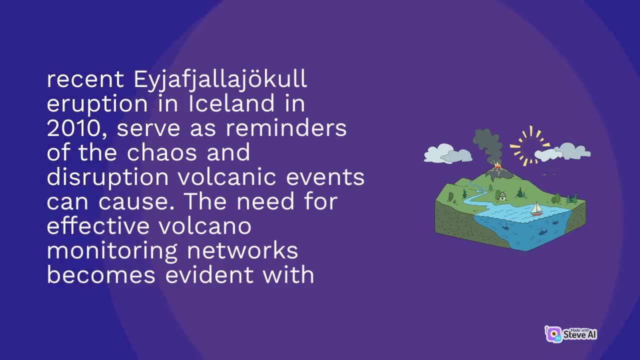 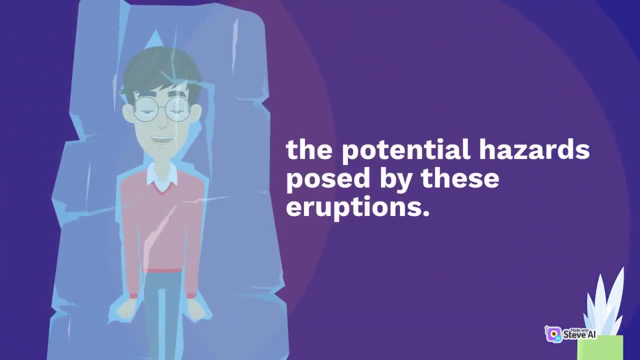 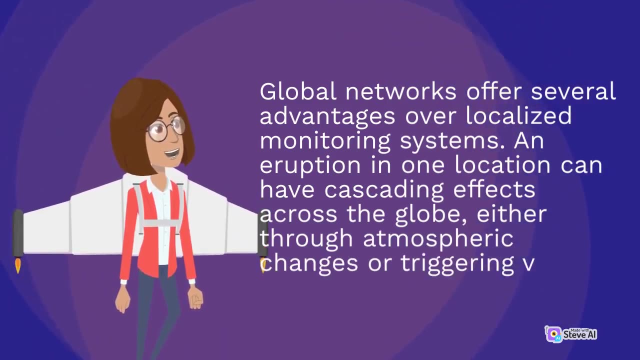 The need for effective volcano monitoring networks becomes evident with The potential hazards posed by these eruptions. Global networks offer several advantages over localized monitoring systems. An eruption in one location can have cascading effects across the globe, either through atmospheric changes or triggering B. 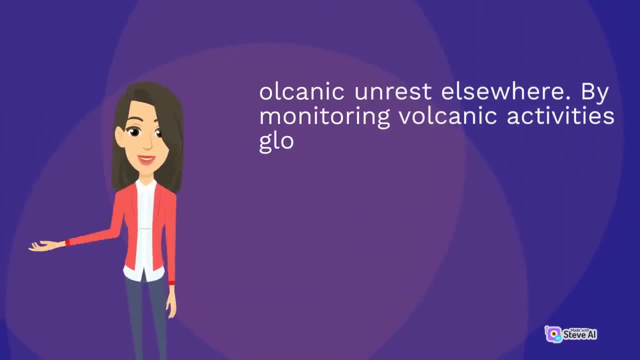 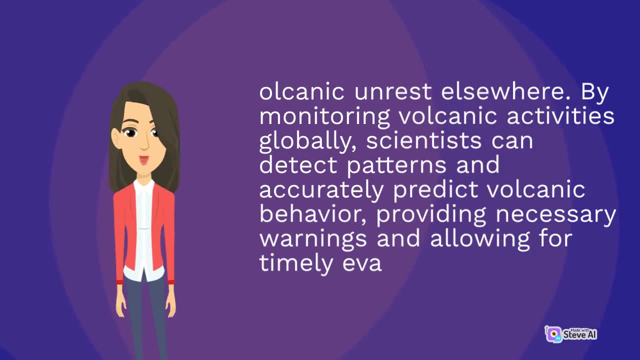 Volcanic unrest elsewhere. By monitoring volcanic activities globally, scientists can detect patterns and accurately predict volcanic behavior, providing necessary warnings and allowing for timely EVA Global networks offer several advantages over localized monitoring systems. An eruption in one location can have cascading effects across the globe, either through atmospheric changes or triggering B. 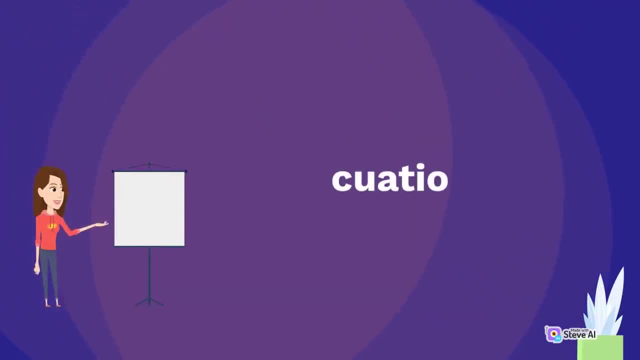 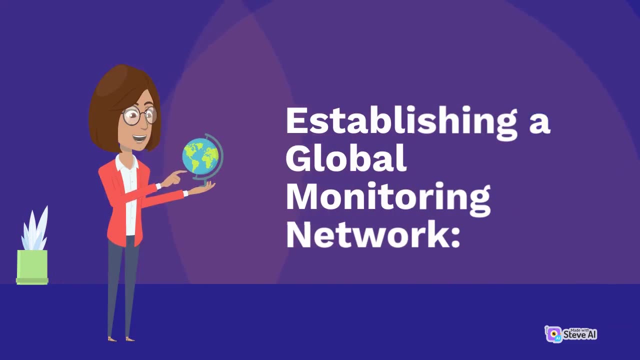 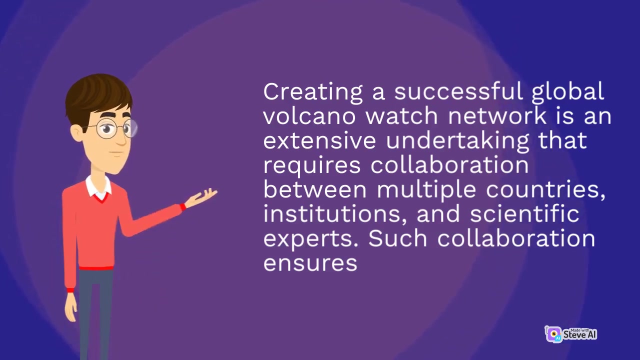 Volcanic unrest elsewhere. By monitoring volcanic activities globally, scientists can detect patterns and allowing for timely EVA Puations. Establishing a global monitoring network- Creating a successful global volcano watch network- is an extensive undertaking that requires collaboration between multiple countries, institutions and scientific experts. 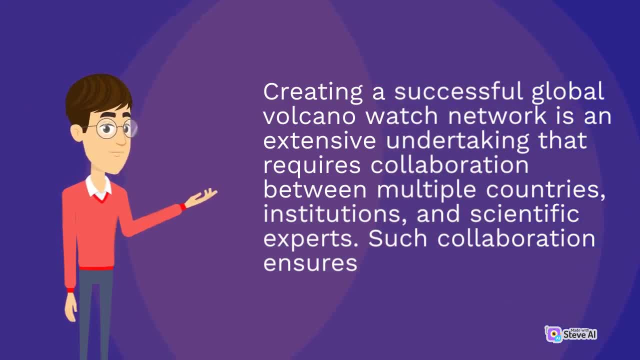 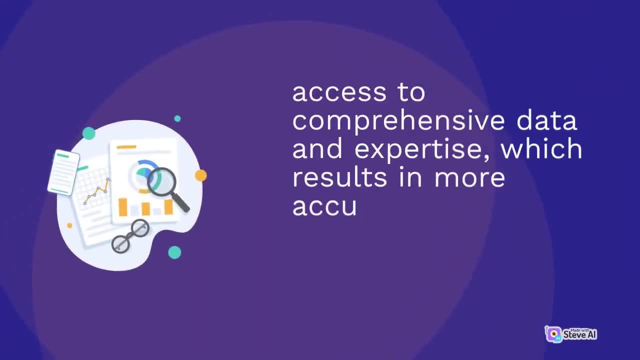 Creating a successful global volcano watch network is an extensive undertaking that requires collaboration between multiple countries, institutions and scientific experts. Such collaboration ensures Access to comprehensive data and expertise in the relevant fields of the research programme, which results in more accurate predictions and improved response measures. 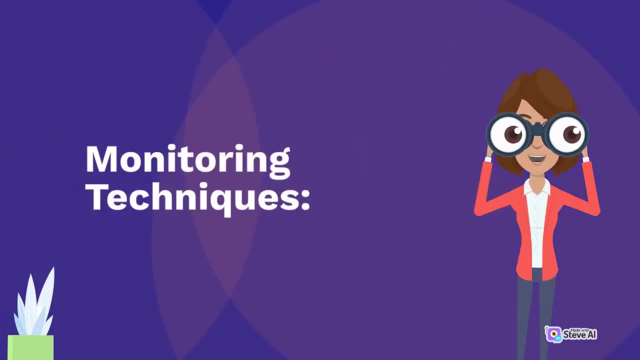 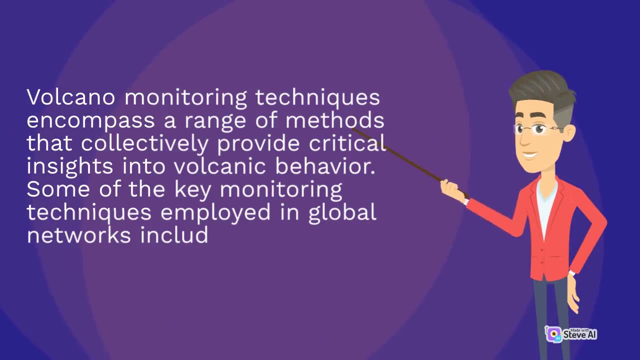 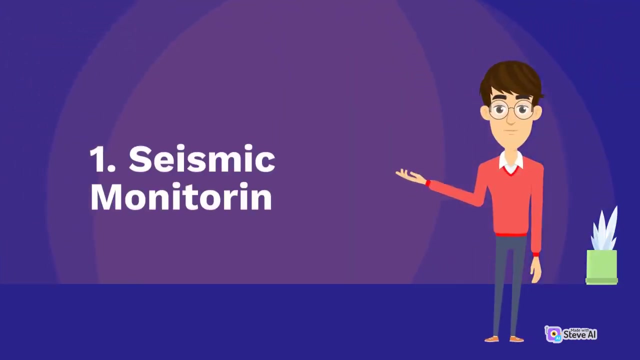 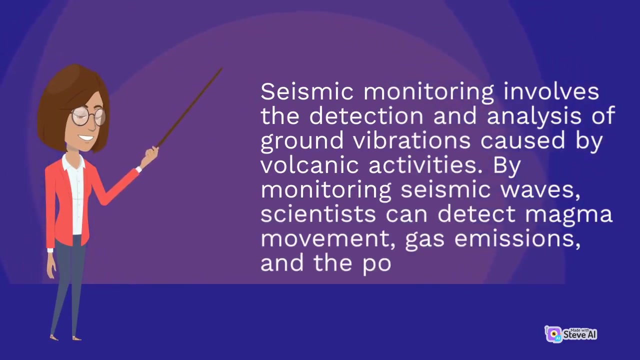 Monitoring Techniques. Volcano monitoring techniques encompass a range of methods that collectively provide critical insights into volcanic behavior. Some of the key monitoring techniques employed in global networks include: E: 1. Seismic Monitoring: Seismic monitoring involves the detection and analysis of ground vibrations caused by volcanic activities. 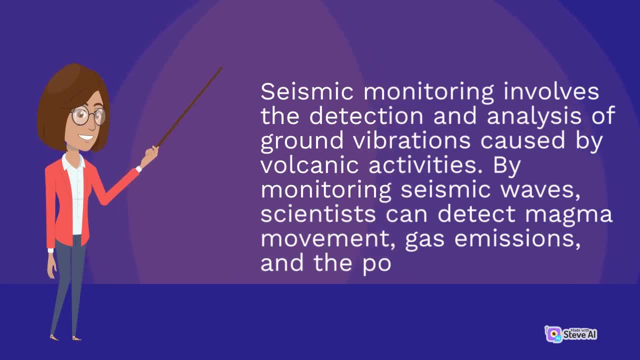 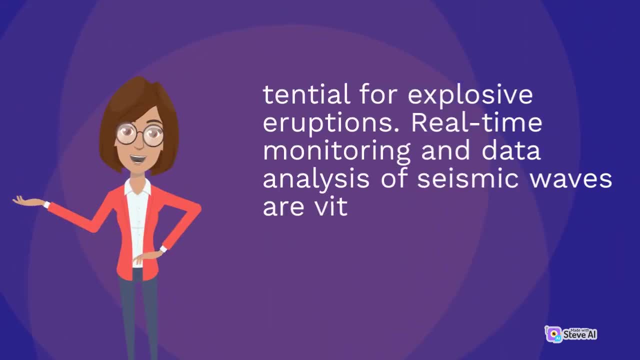 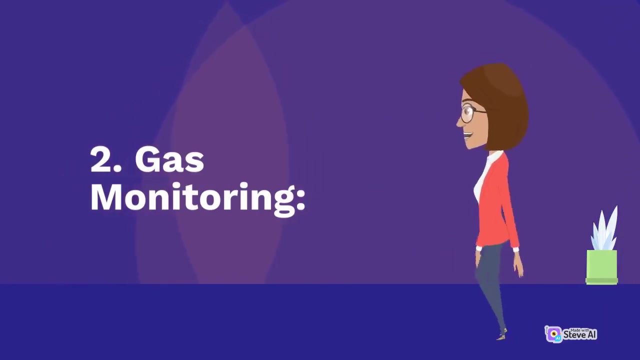 By monitoring seismic waves, scientists can detect magma movement, gas emissions and the POE Potential for Explosive Eruptions. Real-time monitoring and data analysis of seismic waves are vital to providing advanced eruption warnings. 2. Gas Monitoring: Volcanic gases such as sulfur dioxide and carbon dioxide.